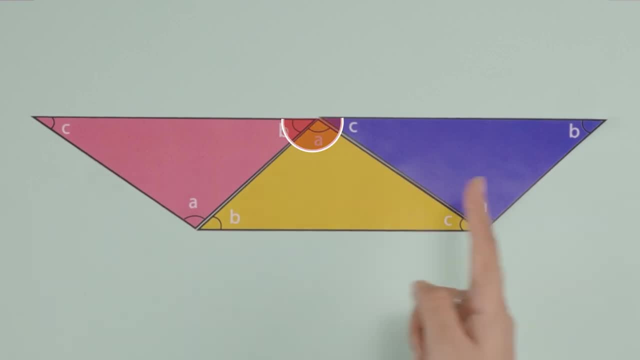 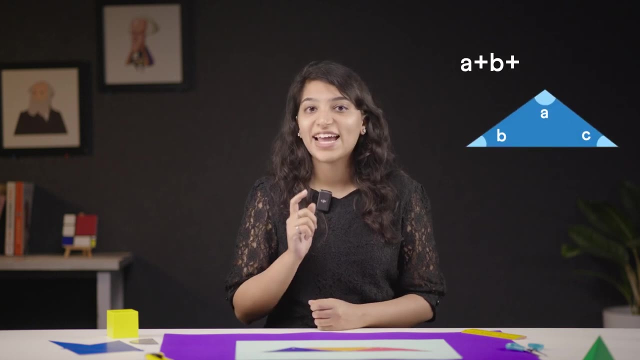 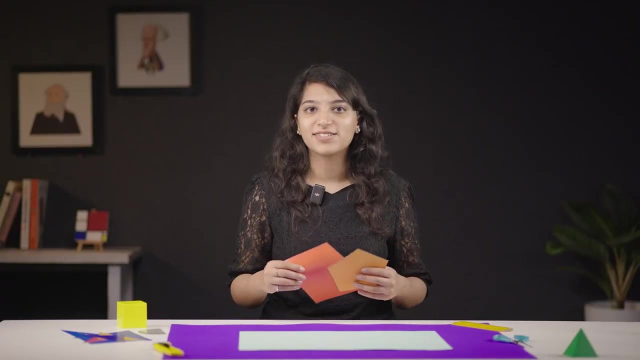 So these three angles add up to a straight angle, making 180 degrees, And that's our visual proof. The sum of interior angles of any triangle is 180 degrees. Now let's use this to find the sum of interior angles of other polygons. 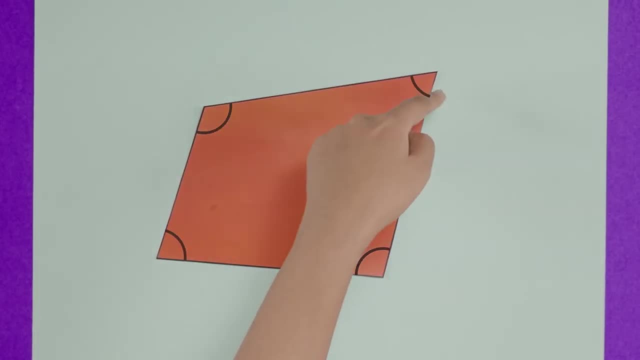 Here's a quadrilateral with its four angles. We can divide it into two triangles. like this: These two angles get divided into smaller angles. Now the three angles of each triangle must add up to 180 degrees. That's a total of two times 180 degrees, or 360 degrees. 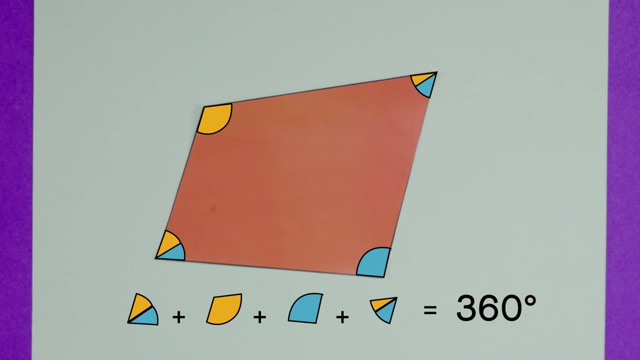 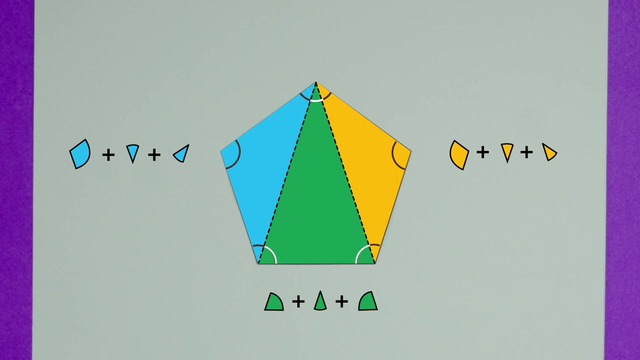 So all these four angles add up to 360 degrees. Here's another polygon, a pentagon, with its five angles. By joining one vertex to the others, we get three triangles. Again, some angles are divided into smaller angles, But what's their sum? In each triangle, the angles add up to 180 degrees. 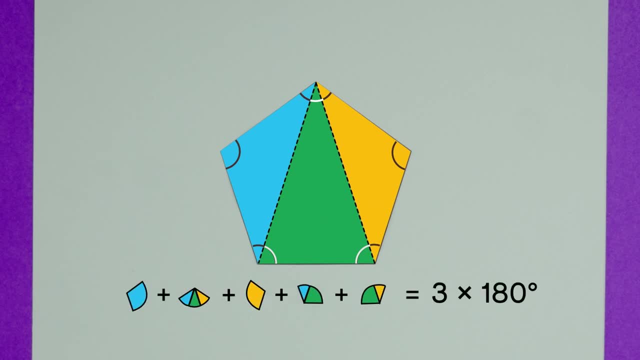 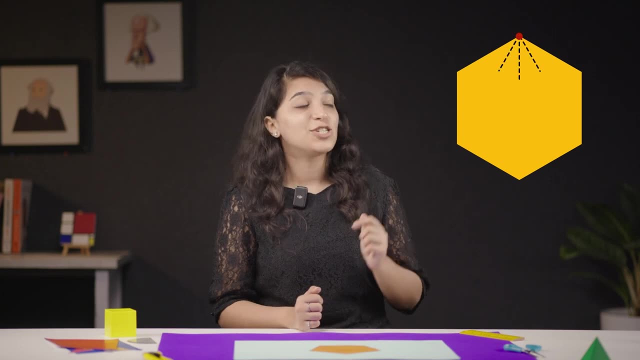 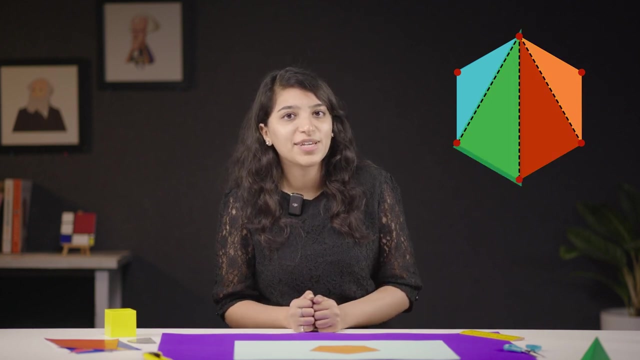 So the sum of all these angles must be three times 180, which is 540 degrees. We can do the same with any polygon. Just take any one vertex and join it with all others. This way we can divide it into triangles. But how many triangles will we get? 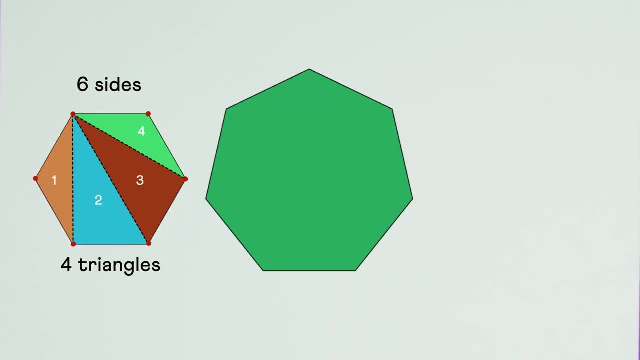 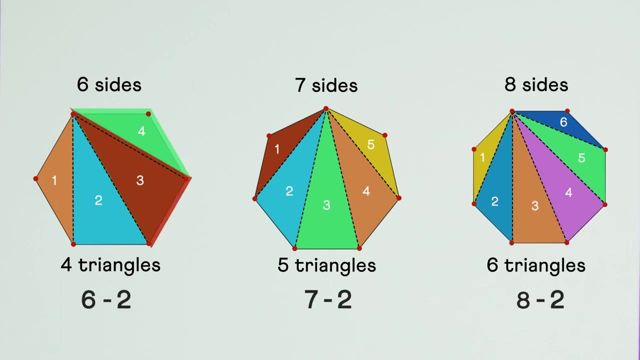 A hexagon with six sides gives four triangles. A heptagon with seven sides Five triangles. An octagon with eight sides Six triangles. The number of triangles are always two less than the number of sides of the polygon, And what's the sum of their angles? 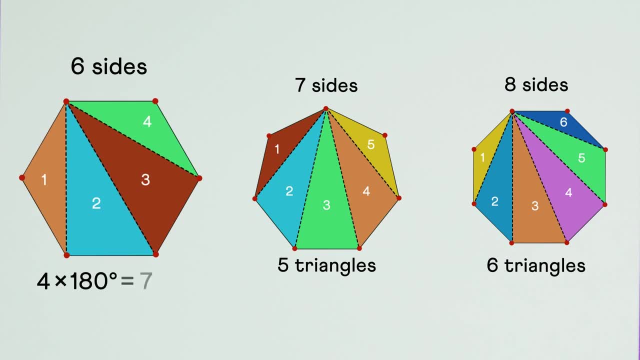 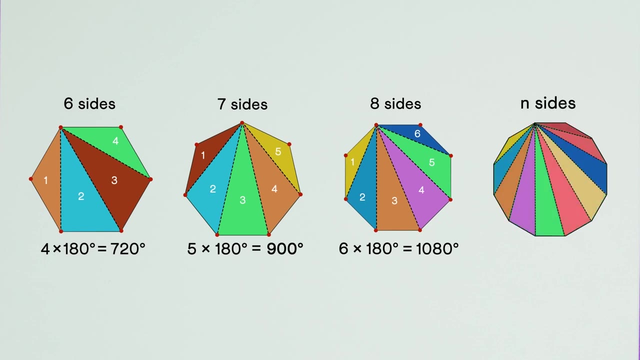 For a hexagon, that's four times 180, 720 degrees. For a heptagon, five times 180, 900 degrees. Similarly, for an octagon, that would be 1080 degrees. So any n-sided polygon can be divided. 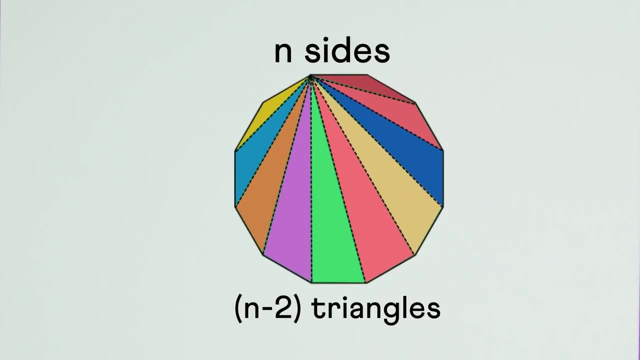 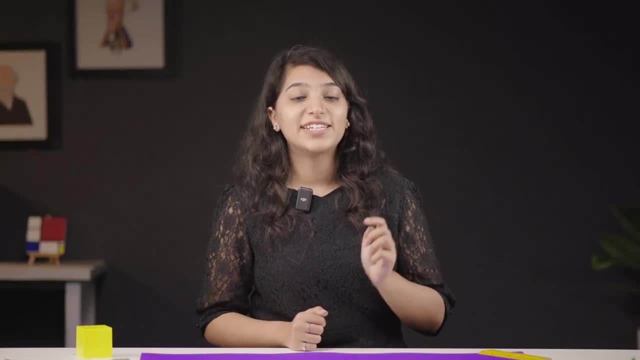 into n minus 2 triangles and the sum of its angles must be n minus 2 times 180 degrees. Now, using this, can you find the sum of interior angles of a decagon that is, a 10-sided polygon? Let us know in the comments.